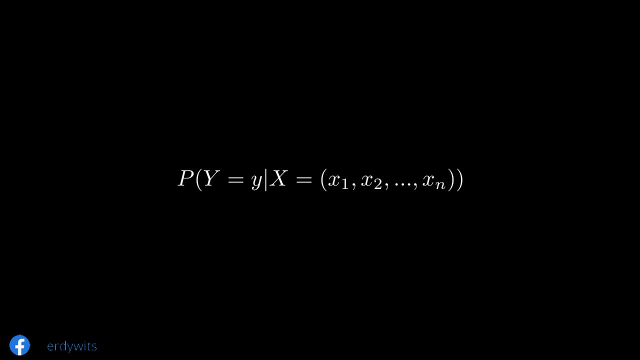 of capital Y is equal to lowercase y, given that capital X is equal to this set. To be more precise, we need to find the particular value of lowercase y for which conditional probability becomes maximum. Why? Because in that case we will be able to say that: 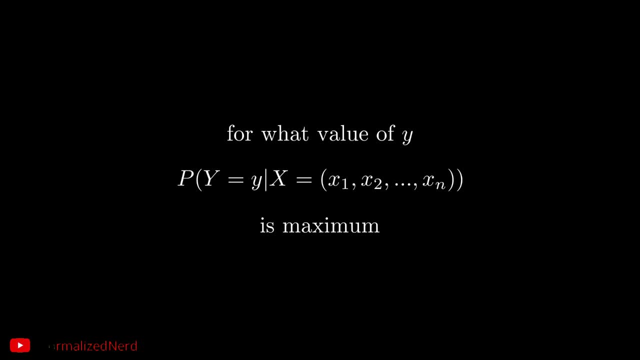 okay, for this particular value of y the expression becomes maximum. So the class label should be this. But the problem is, it is hard to find the probability of y given x directly. To tackle this problem we use Bayes theorem. Yes, this is the portion where Bayes comes into play. 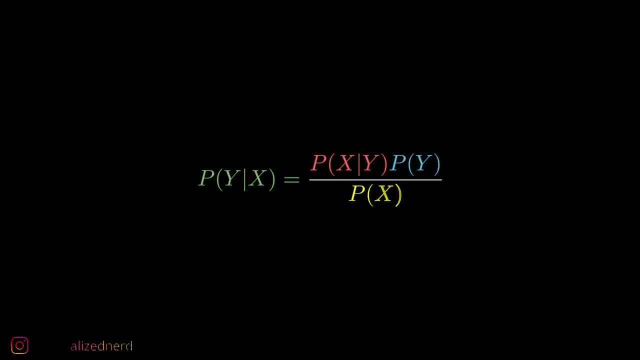 This is the Bayes theorem. It says that probability of y given x that we want to find is same as the probability of x given y times- probability of y divided by probability of x. Now, everything that you can see in the right hand side of this equation can be found from our data set. Let me first tell you how we name these. 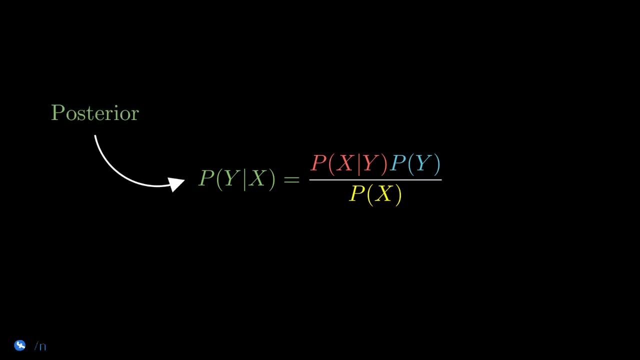 terms, The thing in the left hand side that we want to find is called as posterior, And the thing in the right hand side, probability of y, is called as prior. Why this kind of name? Well, prior means the probability corresponding to an event, before considering any evidence. And 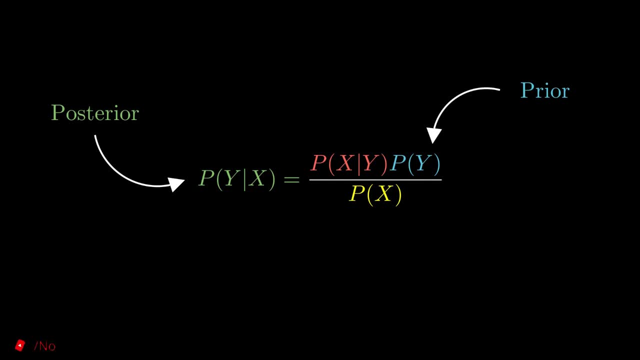 posterior means the probability of that event after considering some evidence. Well, the evidence is nothing but the set of features. So the probability of x is called as evidence here, Because x is just a set of features, right? And the term probability of x given y is named as likelihood. Now here's an. 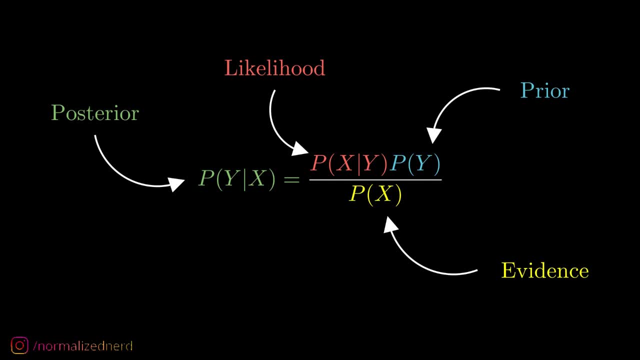 example, The value of the denominator stays the same regardless of the value of y we put in in the numerator, Which simply means to compare the value of this conditional probability for different class levels. we can just ignore the denominator Because the evidence remains the same. To really 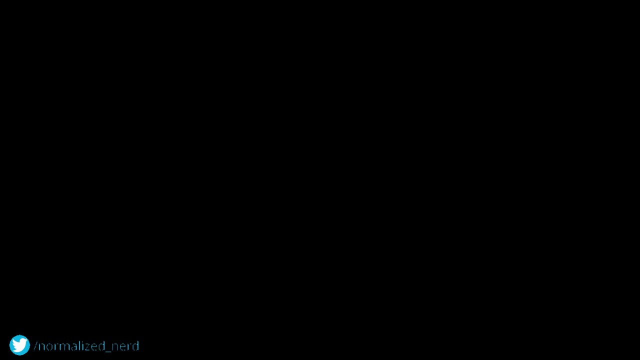 understand the concept, we need to go through an example. Let's consider this small data set. You can see that we have two features: x1 and x2.. And the level variable is y. x1 and x2 can take values from 0,, 1 or 2.. That means both x1 and x2. 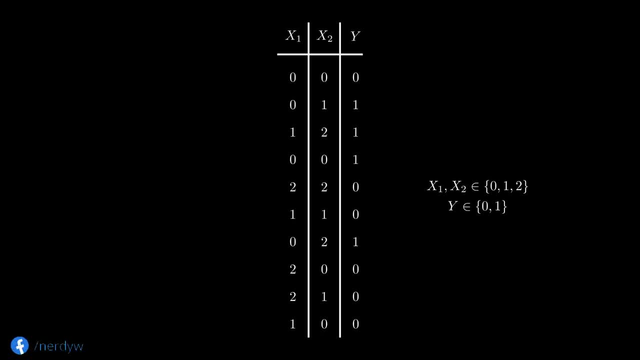 are categorical variables- Well, I will talk about continuous variable later in the video- And y can take two values: 0 or 1. So essentially it's just binary classification. Now imagine that someone is asking us to estimate the value of y, given that x is equal to 0, 2.. That means x is equal to 0, 2.. 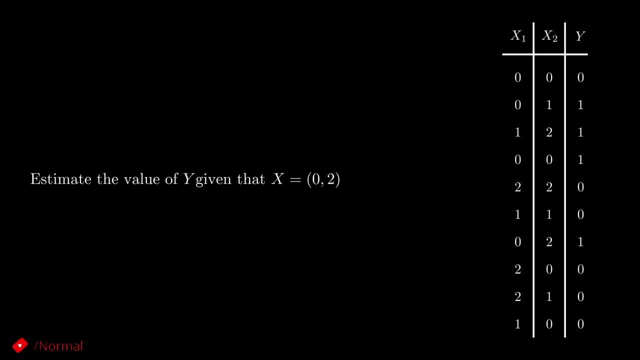 That means somebody has given the value of x1 and x2, that are, 0 and 2, and they want us to find the correct label for that set of feature. Ok, Let's compute the value of the conditional probabilities for both the labels, That is, y is equal to 0 and y is equal to 1.. 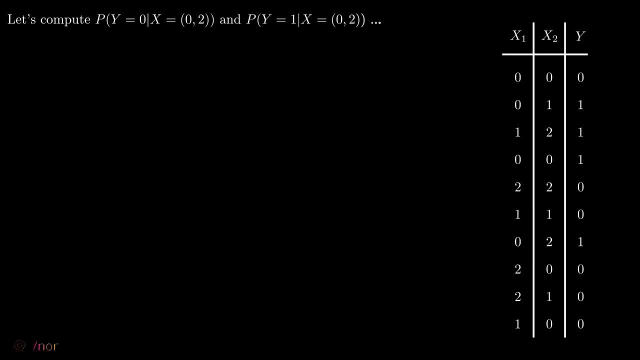 First of all I am gonna compute the prior. That means probability of y is equal to 0 and the probability of y is equal to 1.. So the formula is very simple. In the numerator I am gonna write the frequency of y is equal to 0 and in the denominator 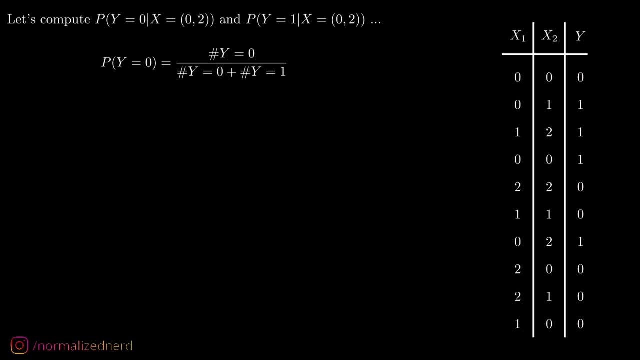 I have to write the total number of occurrences. Now look at the data set. Well, here I have: 6 occurrences of y is equal to 0, and 4 occurrences of y is equal to 1.. So the value of p will be 6 upon 10.. 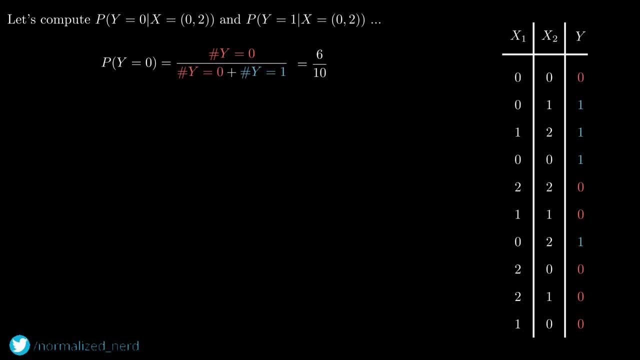 Now to calculate the probability of y is equal to 1, we just need to replace the numerator with the frequency of y is equal to 1, and this is going to be 4 upon 10.. Okay, so we have got our priors ready. 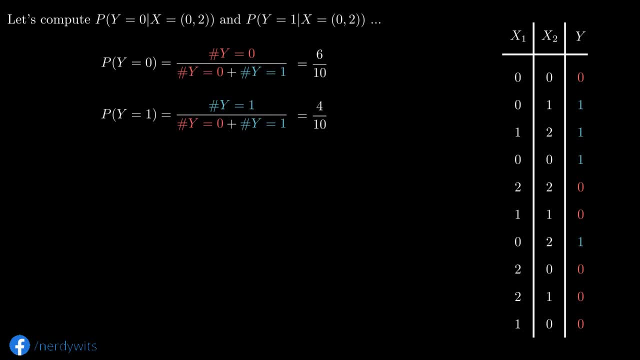 Now let's compute the likelihoods. First I am gonna compute the probability of x, given y is equal to 1.. We just need to look at all the rows where the value of y is 1 and the feature combination is 0, 2.. 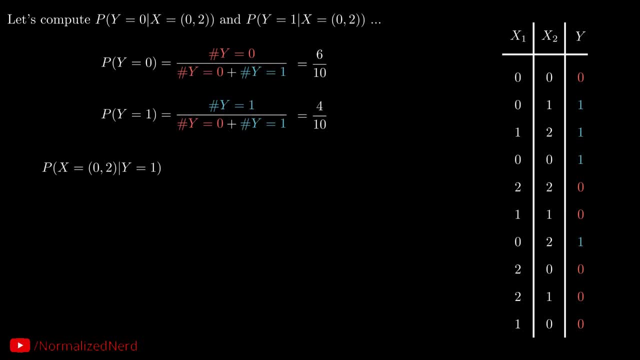 So you can see we have got only one such entry in our data set, So the value of this expression will be 1 upon 4.. Similarly, let's calculate the likelihood for y is equal to 0 and you will see that in our data set there is not a single occurrence where the value of y is 0 and the feature 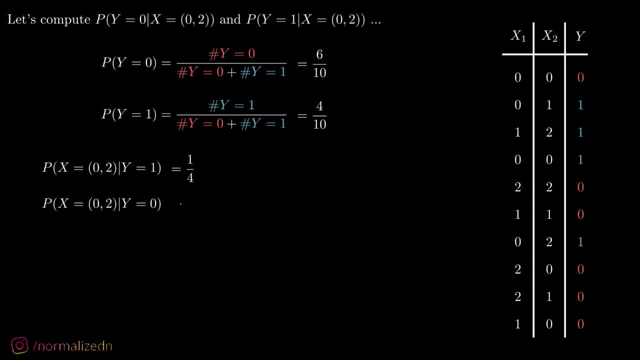 combination is 0, 2.. So the value of this likelihood is 0.. Now to find the class level that maximizes the posterior probability, we just need to compute the numerator that I showed earlier. So the way to do is just by multiplying likelihood y. 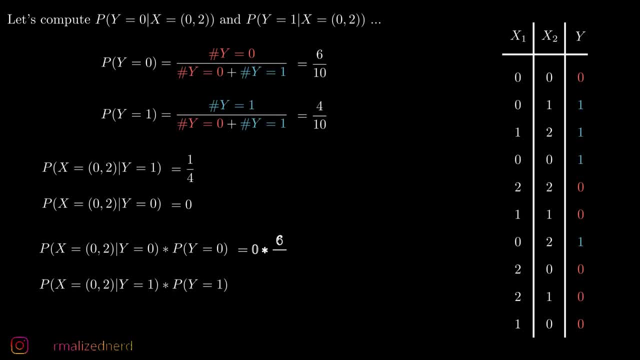 And the likelihood with prior After computing, we see that for the class level 0, the value of the numerator is 0. And for the class level 1, the value is 1 upon 10.. So obviously the class level 1 maximizes our posterior probability. 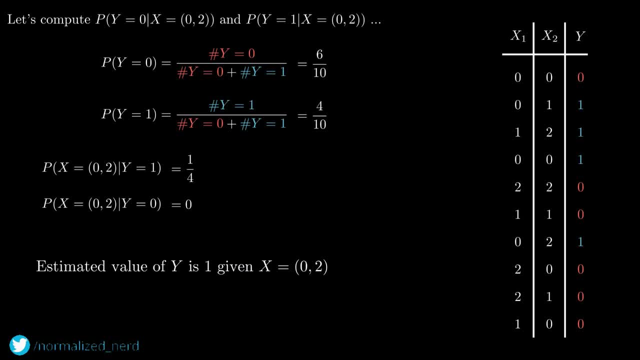 Okay, so we got an answer, So we should be fine with that, right? Well, no, There is a huge problem with this method. The problem is it is hard to find that particular combination of x1 and x2.. As you can see that we only find one occurrence of the instance where y is equal to 1, x1. 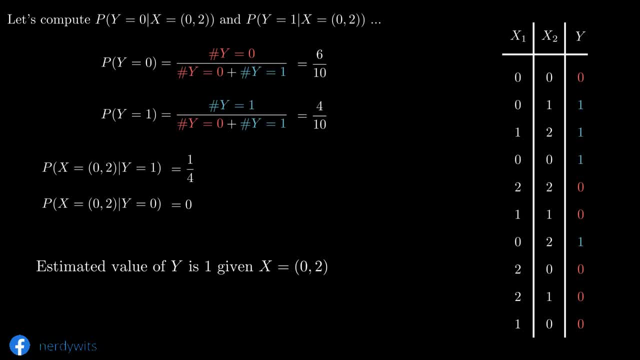 was 0 and x2 was 2.. And we didn't find a single occurrence where y is equal to 0 and x1 is equal to 0 and x2 is equal to 2.. And this is only for 2 features. 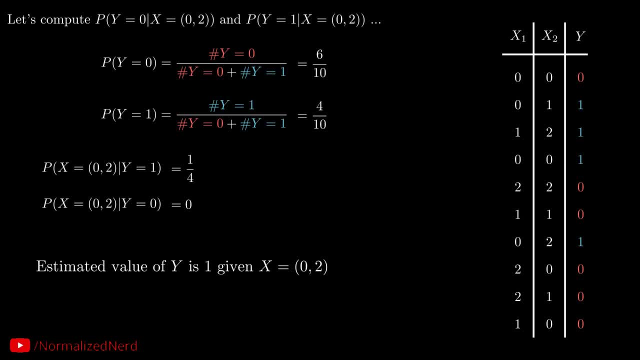 Suppose we have 50 features. So just imagine how hard it will be to find that particular combination of 50 features. Okay, If we have 50 features in our dataset, it is very likely that we will never encounter some particular combination of features, right? 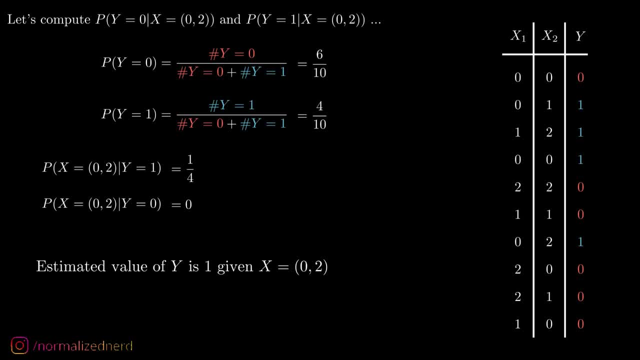 And if we don't find even a single occurrence of multiple such combinations, then the probability value will always be 0. And we can't really compare if we have multiple 0 values right. So to tackle this problem, we use naive Bayes classifier. 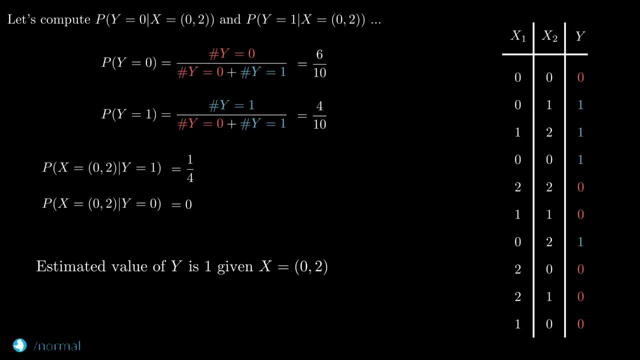 Well, the concept is very simple. We just need to consider that x1 and x2 are independent of each other. Now why this can help. Well, if we just consider that x1 and x2 are independent of each other, then we don't need 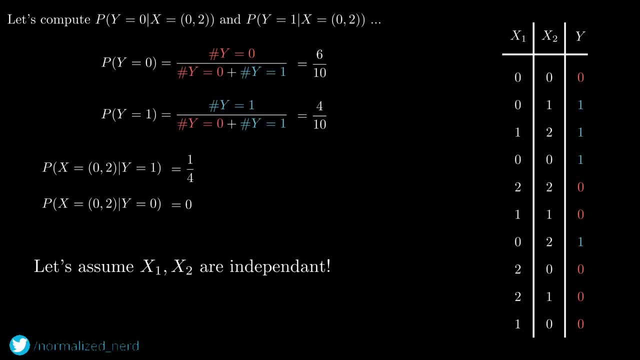 to actually find that particular combination of x1 and x2 in our dataset. We can just write the probability of x given y as a product. Let me show you, Please understand, that We wouldn't be able to write this if the features are not independent. 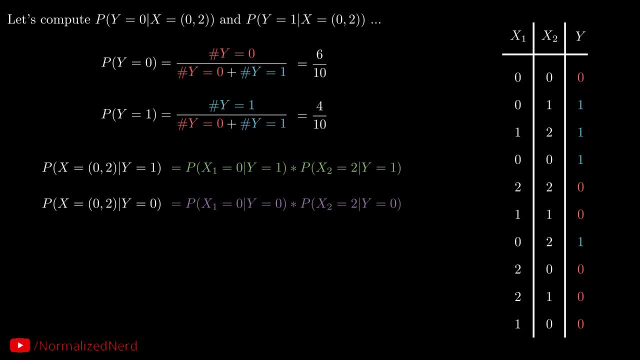 So that's the big assumption that naive Bayes makes. To be honest, in real worlds the features might not be actually independent. That's why it's called a naive approach towards the problem. But it makes our work easier and it produces really good results. 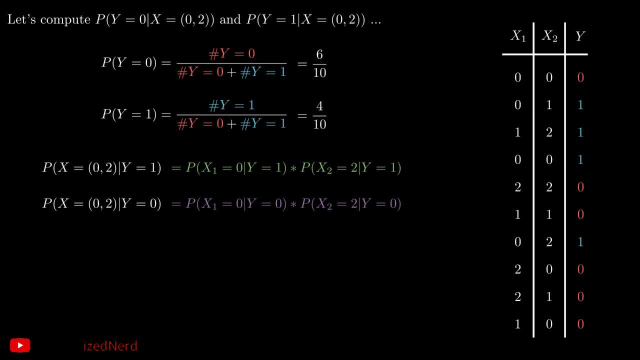 So let's first compute the probability of x1 is equal to 0, given y is equal to 1.. Well, to do this, we just need to count the entries where x1 is equal to 0 and y is equal to 1 and x1 is equal to 0.. 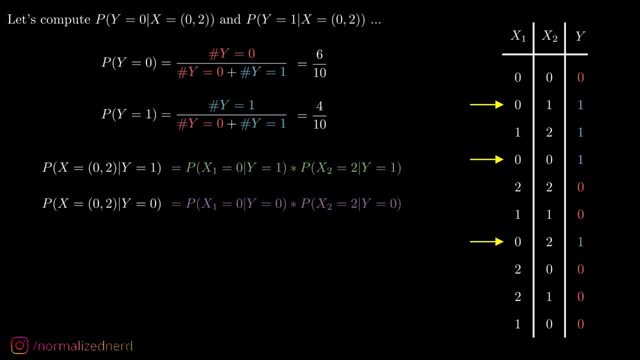 So, as you can see, there are three such cases and the number of occurrences where y is equal to 1 is 4.. So the probability will be 3 upon 4.. Similarly, if we calculate, the probability of x2 is equal to 2, given y is equal to 1,. 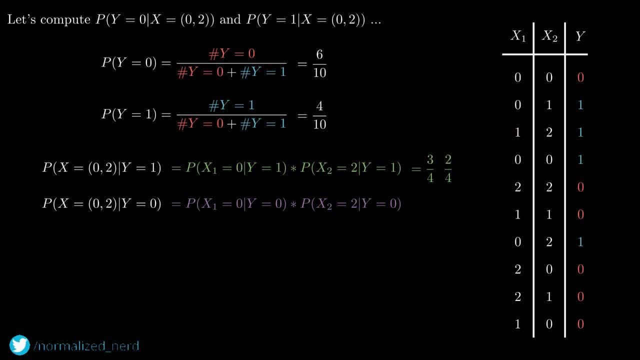 we will get 2 upon 4.. Now let's come to the next line. So here, first we need to find how many times the value of x1 is equal to 0 where y is equal to 0. If we find out, there is only one occurrence and the number of cases where y is equal to. 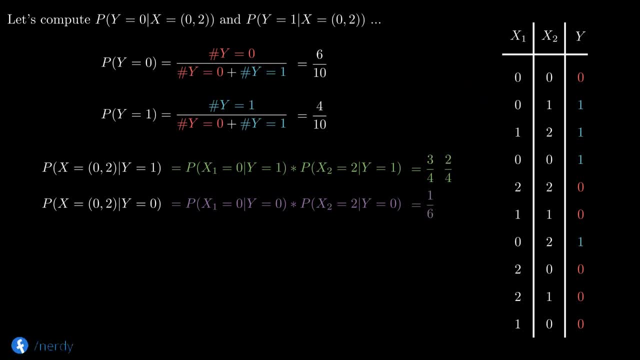 0 is 6.. So the probability becomes 1 upon 6.. Similarly, if we calculate the number of cases where x2 is equal to 2 and y is equal to 0 is 1.. So here also I'm gonna have 1 upon 6.. 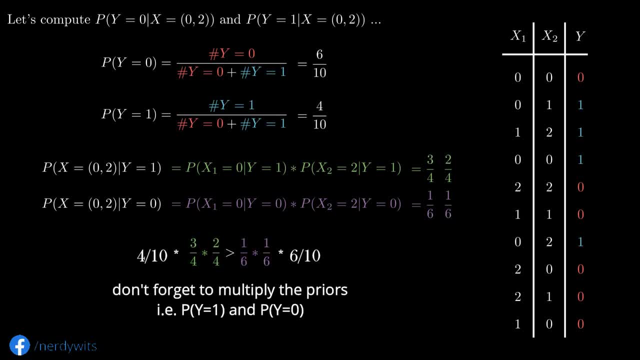 Now let's compare them. So obviously the first probability is greater than the second one. So we can clearly see that The class level 1 maximizes our posterior probability. So the estimated class level is 1.. And voila, Now you know how Naive Bayes works. 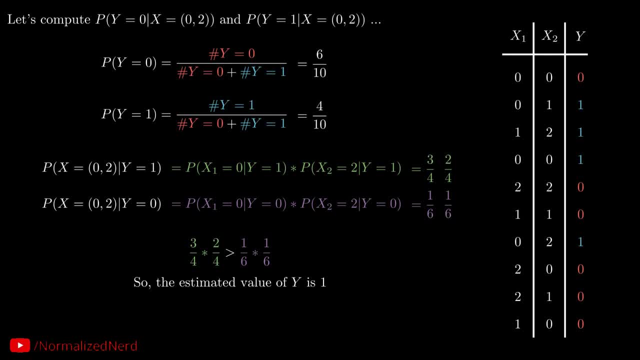 Okay, so now I'm gonna talk about how you can deal with continuous features. So until now we were dealing with categorical variables, right. x1 and x2 were both categorical And in that case we could actually compute the frequencies. But in case of continuous features we can't compute the frequencies, right? 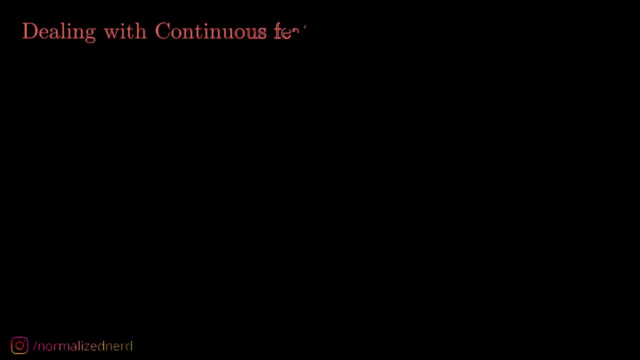 So how to tackle this? Well, there are many ways. I'm gonna discuss two ways. The first one is discretization. Suppose there's a continuous variable named age And let's consider that the value of age lies between 11 and 50..